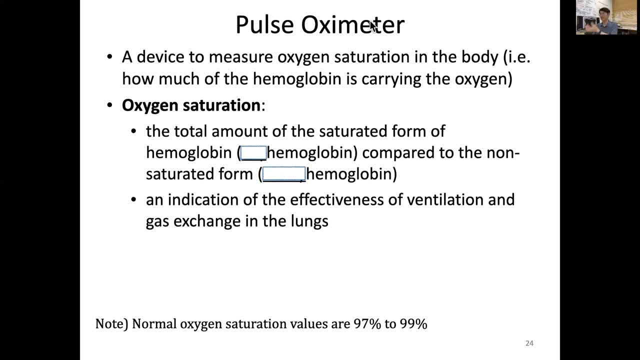 called pulse oximeter, So oxygen meter measurement. So oxygen saturation is the total amount of saturated form of hemoglobin, or we call oxyhemoglobin, compared to non saturated form or deoxyhemoglobin. And this oxygen saturation is an indicator of effectiveness of a person's 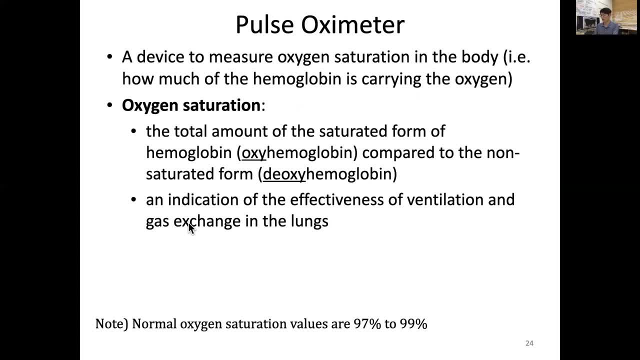 ventilation and gas exchange in the lungs. So let me give you a formula. So that's a percentage of a saturation of oxygen is, you know, oxyhemoglobin divided by total hemoglobin C concentration, and total hemoglobin is composed of oxy and deoxyhemoglobin, and 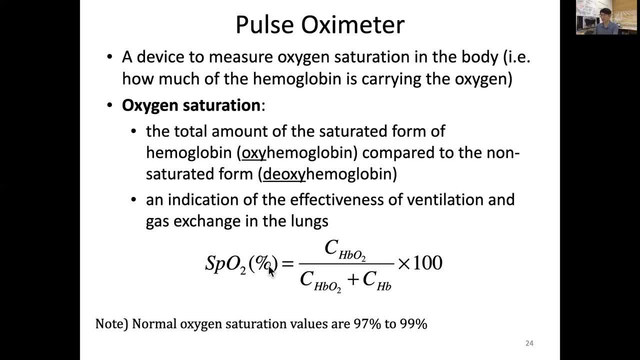 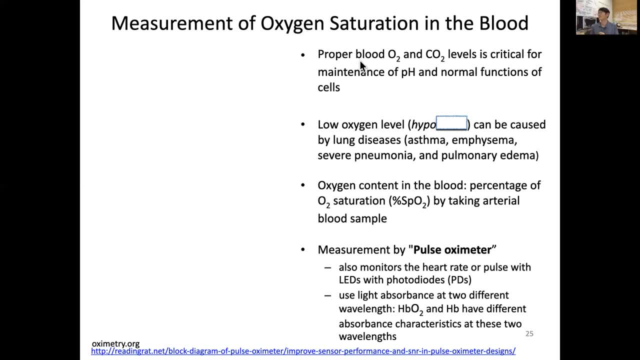 multiplied by 100 for making percent. So to measure this oxygen saturation in the blood, the proper blood oxygen, co2, which is crucial for maintaining our pH and normal function of our cells, So to measure we use a trick based on biophotonics and the optical property of the blood. You. 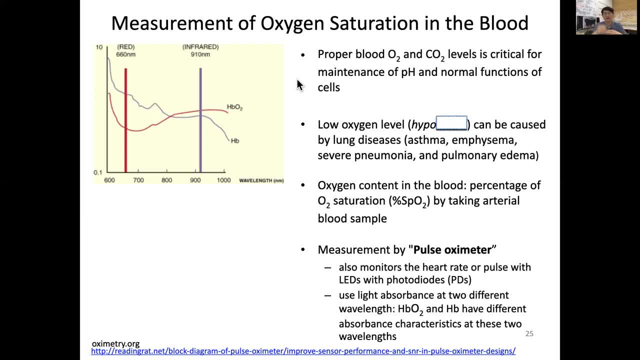 remember that some blood, when you cut, you can see a dark, darker color of blood. but if you happen to have a, let's say, a real arterial blood coming, that's a bright red. So the different color means something and that using that difference in color or the color means the absorption of 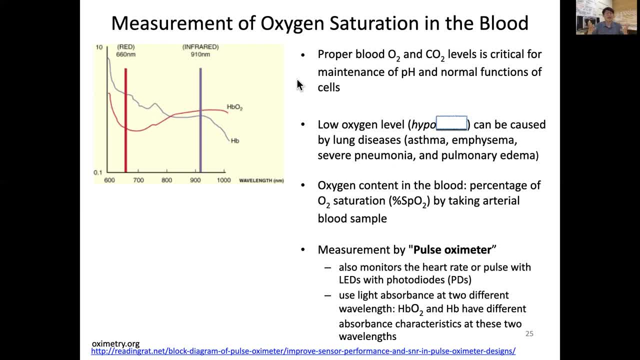 the light in visible ranges are different And using that we could actually quantify a, the status of oxygen saturation. So that's showing up in this absorption spectrum. what it means is you see this x-axis as a wavelength or color of the light and y-axis is the absorption, So you can see bloods are. 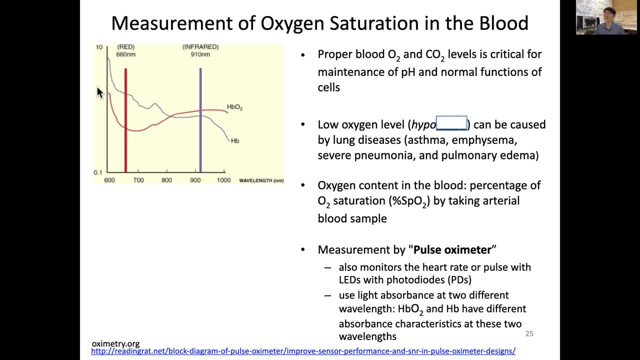 usually are red because this high light is the absorption of oxygen. So this is the absorption of oxygen. So you can see bloods are usually red because of this high absorption in the green and blue range. and interestingly, the oxy deoxy hemoglobin has quite different absorption and you can see oxy hemoglobin has much lower in. 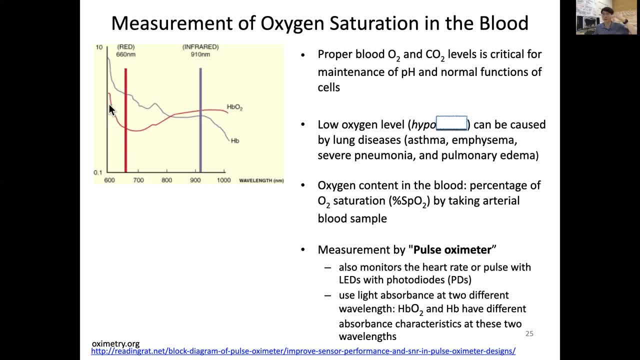 this 600 to 700, which is red color. absorption is low. what that means is red color. when hit this hemoglobin it will reflect more. that's why in our eye it looks bright red color. so that's oxy, hemoglobin spectrum and deoxy. so in 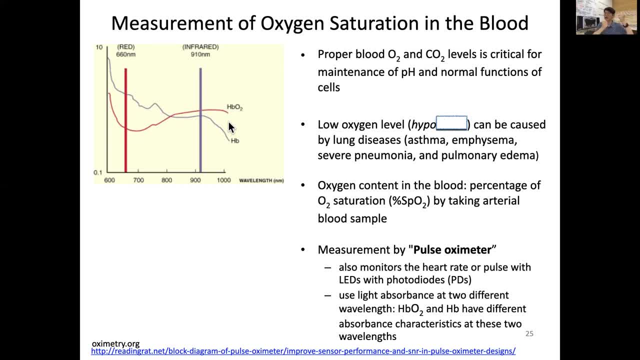 principle there's only two unknowns: concentration. so you could just use two colors of of light sending through the tissue and detect, and you can recover the concentration of two variables. so that's the trick: low oxygen level or hyporoxy, cyclin, cyclin Hypoxemia. Semia means in the blood, oxygen in the blood is low, hypoxemia. 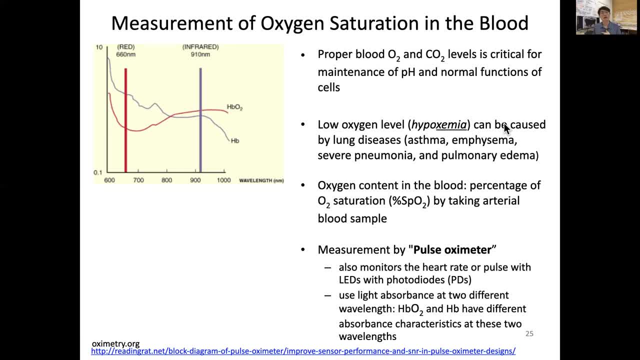 So low oxygen level it can be caused by lung underlying disease such as asthma and emphysema and severe pneumonia and pulmonary edema. All of these affect airway and lung parenchyma, which will affect our proper oxygen gas exchange. 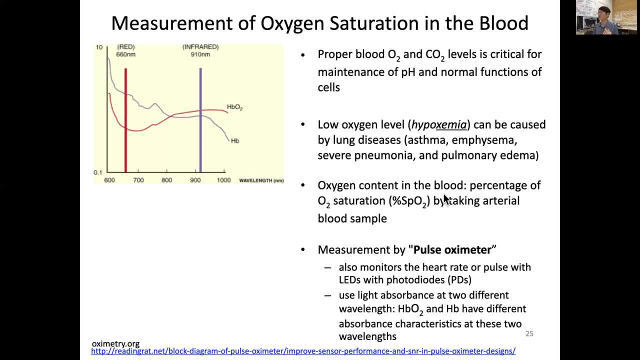 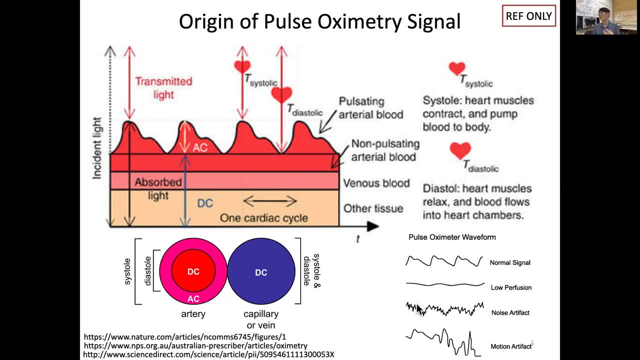 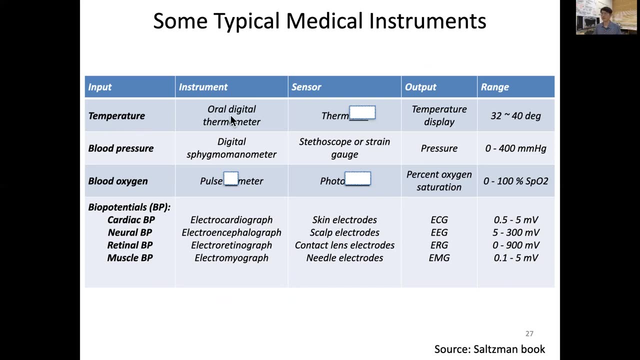 so it gives us an engineering challenge and problem to how to analyze this signal and turn it into a oxygen saturation percent. So now I want to summarize typical medical instruments and example temperature. I show oral digital thermometer which uses a thermistor as a sensor, and that output. 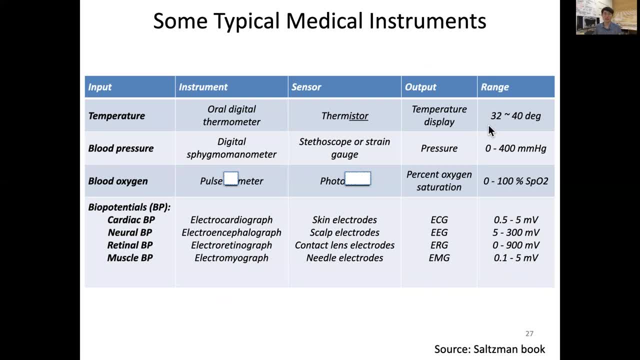 will give a temperature within the range of 32 to 40 degree Blood pressure, as a simple one now has a digital spectrometer and the sensors are stethoscope or strain gauge and the output pressure is 0 to 400 millimeter Hg and blood oxygen. we use pulse oximeter and that sensor was a 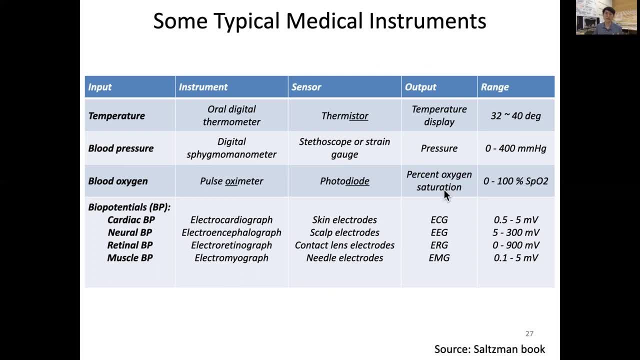 photodiode and that gives a percent oxygen saturation from 0 to 100 percent. So now I want to show you how to use a thermistor as a sensor and that gives a, and electrical sensors, which I haven't discussed much, but that's called. 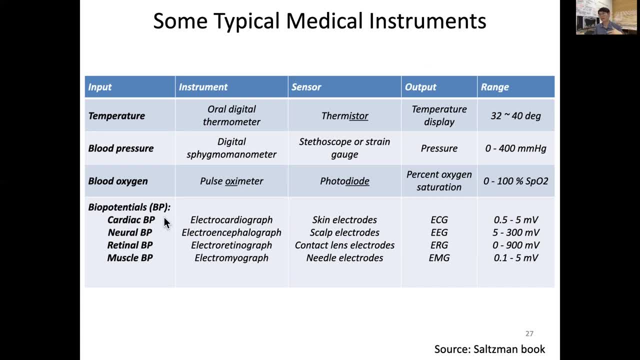 biopotential, and there's cardiac biopotential, neural, retinal and muscle, and that's we call electrocardiography, electroencephalography or EEG, and electroretinography and electromyography. and you can see there are different kind of skin, scab, contact lens and needle electrodes and that's. 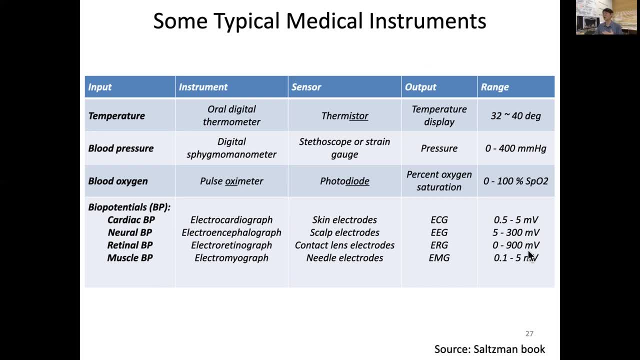 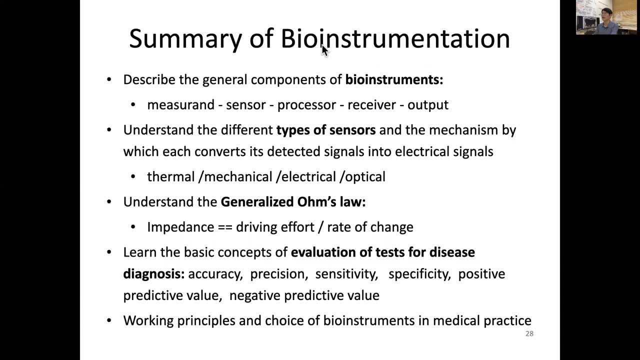 uh, measuring the range of a millimeter to several hundred millivolt which is happening as a biopotential inside our body. So in summary of bio instrumentation, we describe the general components of bio instruments as the measurement parameter and we use sensor and we process it to receiver to display as an 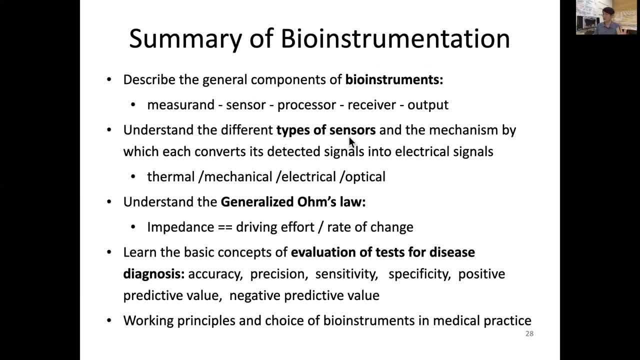 output and we have to understand different type of sensors and the mechanisms of principle Which converts its detected signal into something useful for us. that is usually electrical signals and we just discuss a thermal, mechanical, electrical and optical sensors and I also discuss about generalized ohms law, that all these uh, different types of mechanical translational